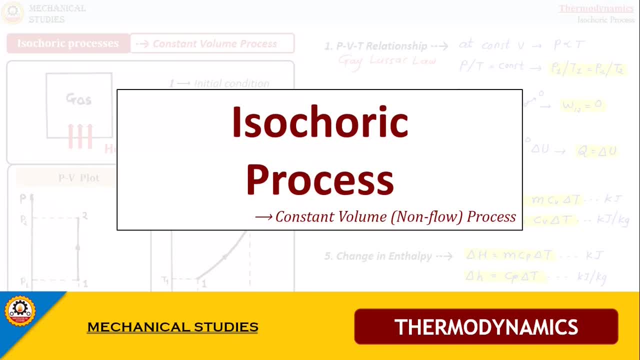 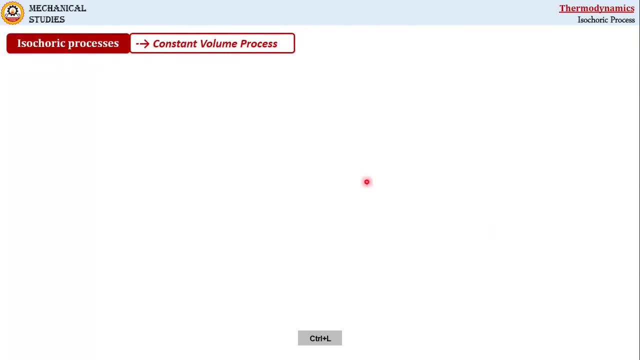 steady flow processes. Okay, so let's begin. Isochoric process is a constant volume process during which the volume of working substance remains constant, while other properties of working substance vary. Okay, to understand this, let's consider here an example of a gas enclosed. 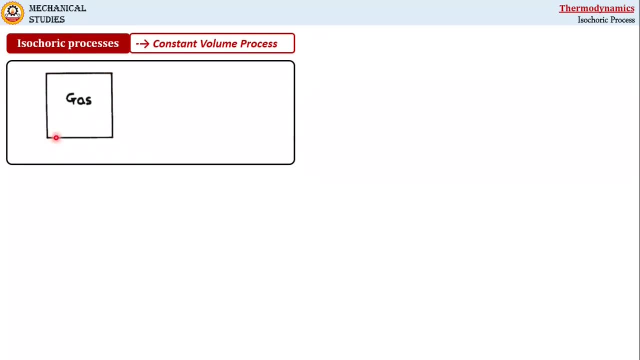 in a rigid system. Let's consider here an example of a gas enclosed in a rigid system. Let's consider here an example of a gas enclosed in a rigid system. Let's consider here an example of a gas enclosed in a rigid tank or rigid container and which is: 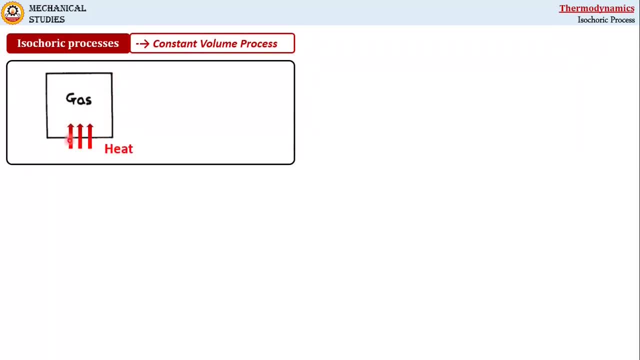 heated by some external source. So as the gas is heated it will try to expand. but since gas is enclosed in a rigid container, the change in its volume will be restricted here, and that will cause the gas to expand. Now let's consider here state 1 as initial condition of the gas and which can be 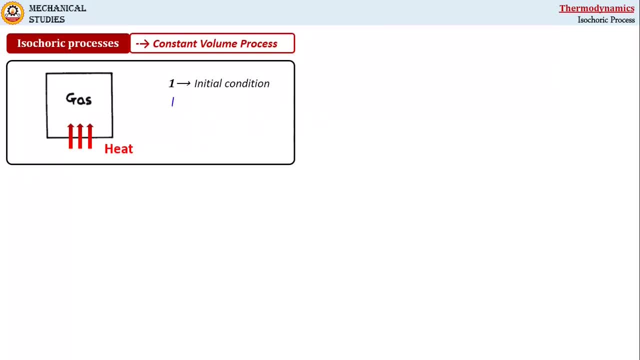 described with the help of properties like pressure P1, volume V1, temperature, let's say T1, and entropy S1.. Similarly, let's consider state 2 as final condition after heating of gas, and that can be described with the help of same properties as pressure P2, volume V2, temperature T2 and entropy. 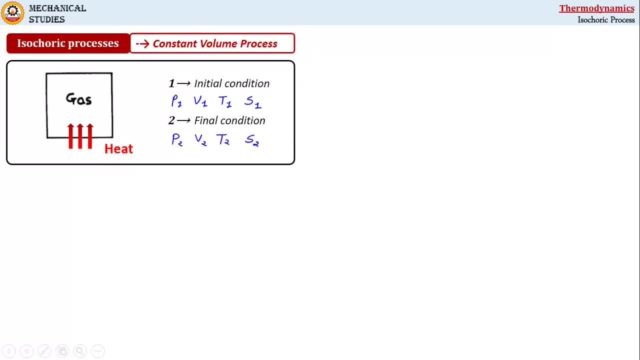 S2.. Okay, so these properties will help us to describe the process of a gas enclosed in a rigid system. Let's consider here a gas enclosed in a rigid container and which can be described with the help of properties like pressure- P1,- volume- V2, temperature- let's say T1- and entropy- S2.. Okay so these properties 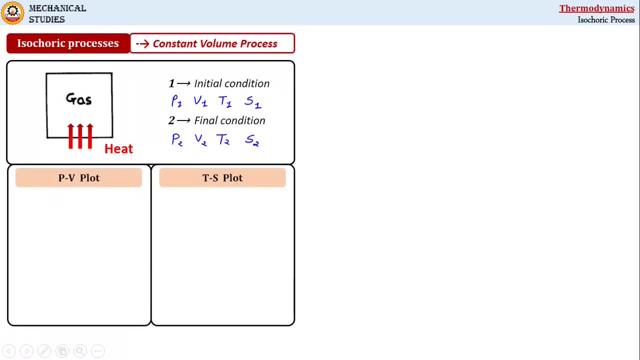 will help us to describe the process of a gas enclosed in a rigid container and which can be described with the help of same properties as the paint glass in a rigid container, and which can be described with the help of same properties as pressure- P1, volume- V2, temperature, let's say T1, and 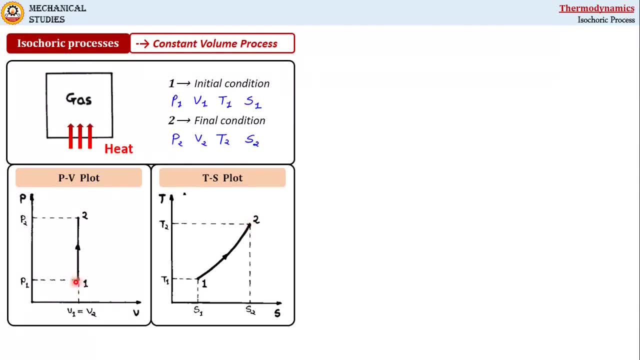 temperature, let's say T2 and all. Finally, there are two properties of color 마음에 spacalling that had only one set of properties in each one and which is call P1, and Now we can see that, lookin at these two properties when we take, consider this and 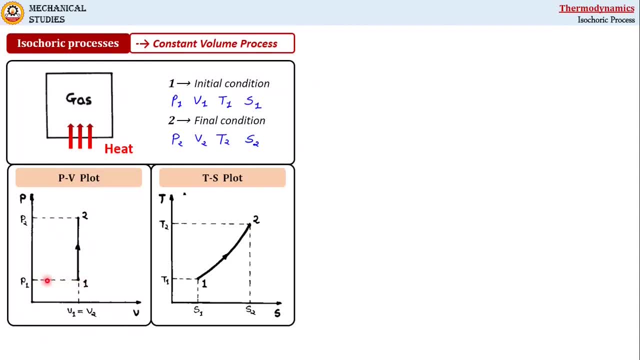 visualize these two properties here. Let's recall that if we look at 1 and two, we'll get that the heat soil size of the gas is equal to the volume of gas, which represents the sameền33.側. and when you multiply this valueичесque value, иyan dv, when we beep the 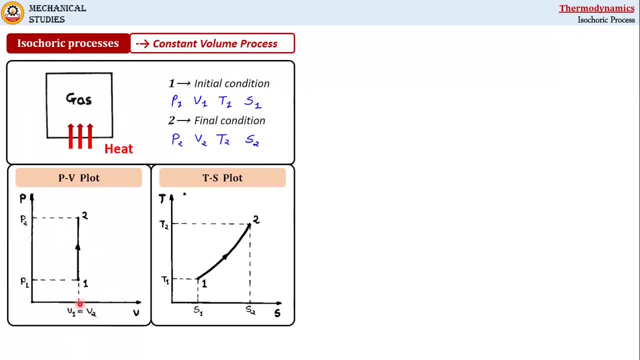 3.5 or less value of вам 4000 from rn, then the temperature and temperature are equal. If vous watch this video, let me repeat next V2. and that's why this isochoric constant volume process is represented with vertical. 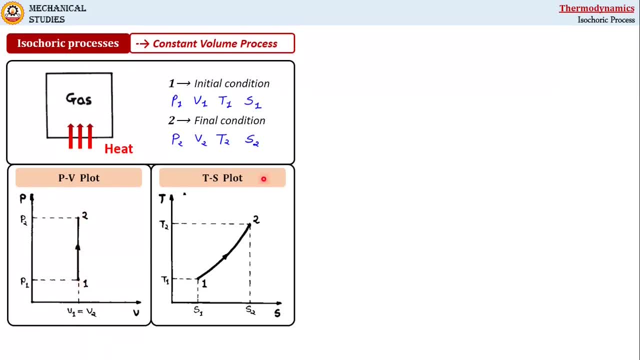 straight line on pressure volume diagram. On temperature entropy plot, the gas is initially at state 1, which is having temperature T1 and entropy S1. So when it is heated its temperature obviously increases from T1 to T2 and on the another side its entropy also increases from S1 to S2.. 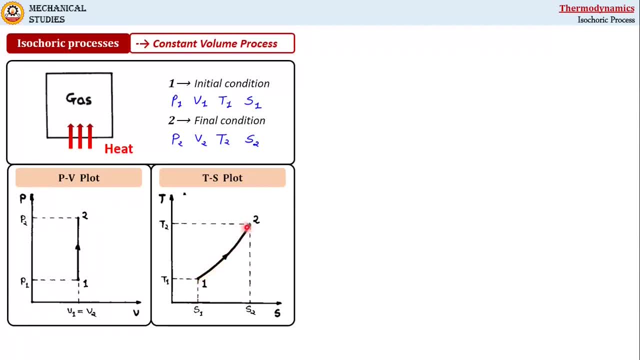 So this isochoric process is represented by this curve 1 to 2 on temperature entropy plot. Now please note here very important point regarding entropy- that whenever you are adding heat to a substance, its entropy increases, And whenever you are Extracting or removing heat from a substance, its entropy will decreases. 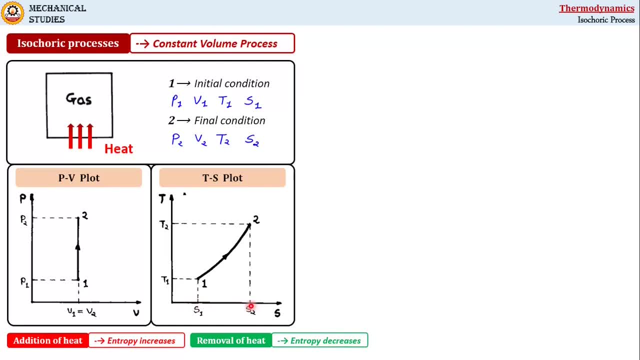 So you can see the effect of heat on this temperature entropy plot. So, instead of heating, if it was a cooling process, then the direction of the process would be simply reversed here like this: If it was a cooling process- constant volume cooling process- then the direction would be: 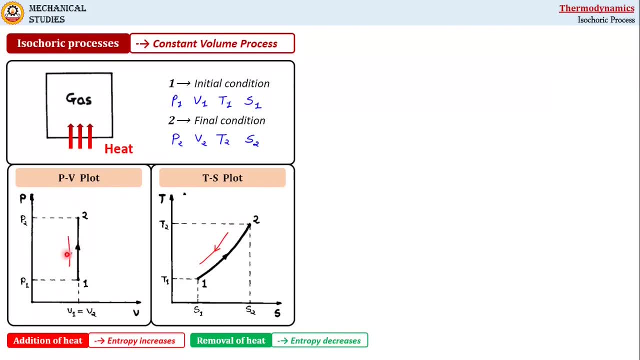 simply reversed. So this, this will be the trend of that process. After pressure volume and temperature entropy plots of this process, we will move forward to pressure volume and temperature relationship. Now, during isochoric process, volume remains constant. It's a constant volume process. 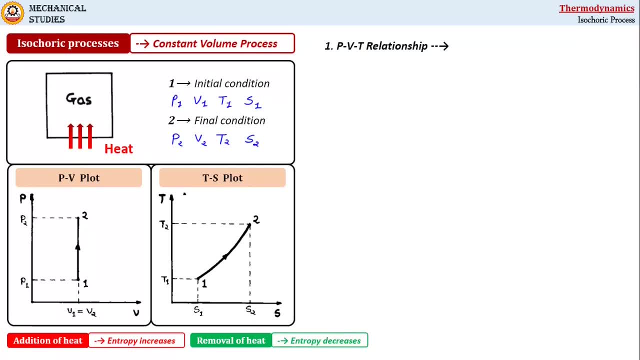 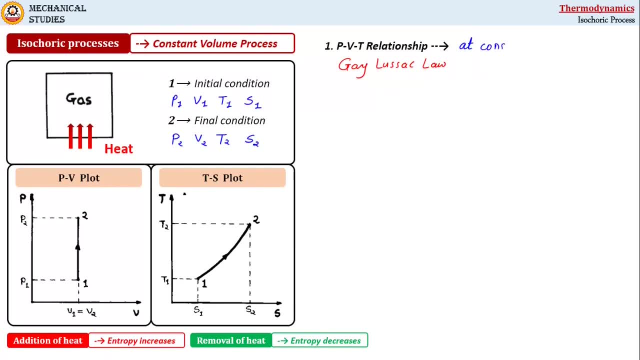 At constant volume. At constant volume, pressure of ideal gas is directly proportional to temperature. So we can write at constant volume. Ratio of pressure to temperature is constant. This is what is HDMI. This is what is volume. constant p by t will be constant. okay, so we can write for process one to two. 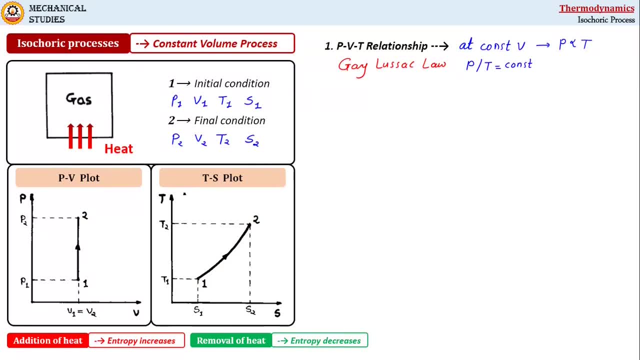 the relationship between pressure and temperature. as p 1 by t 1, this will be equal to p 2 by t 2, p 2 by t 2. so this is the relationship between pressure and temperature for isochoric process. next we will see work done associated with this isochoric process and we know work done. 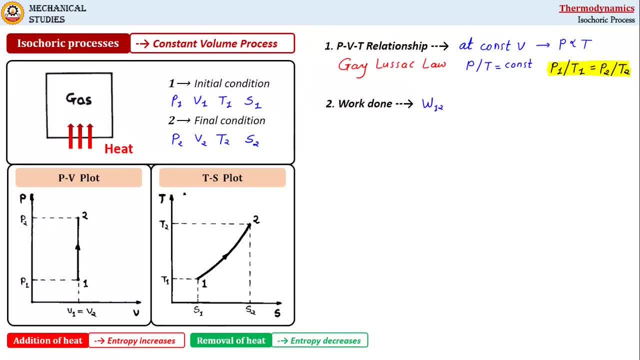 for process. this 1 to 2 can be written as w 1 to 2. it will be equal to integral of del w in between limit 1 to 2. okay, here del w represents moving boundary work and system do not possess any, any any. 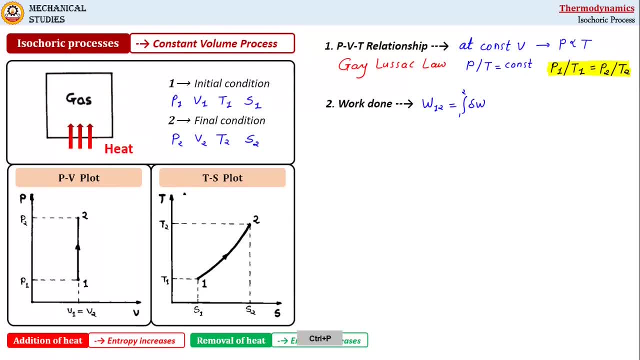 external work interaction. so we can substitute here del w as 1 to 2. this will be integral 1 to 2. del w will be equal to p into dv, which represents moving boundary work. now, here it's a constant volume process and that's why change in volume. 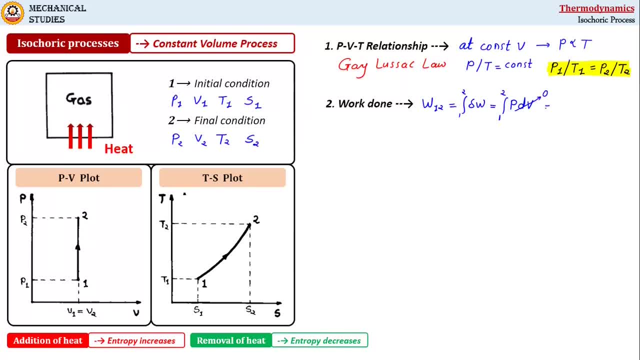 is 0 here. so ultimately this will be equal to integral of 0, and that will be equal to integral of 0 will be constant in between limits 1 to 2, so that will be again constant minus constant, so it will be 0. so here, work done associated with constant volume. 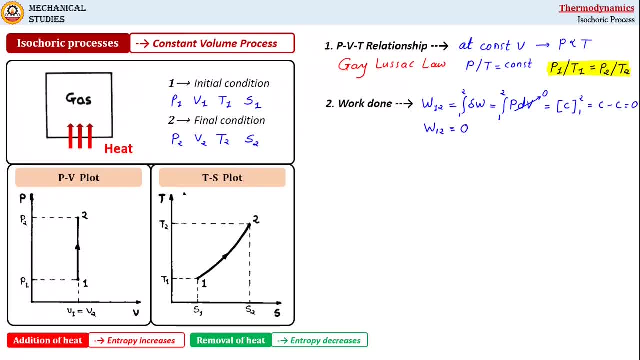 isochoric process will be 0. okay, thus the work done for non-flow isochoric process is 0. now we will apply the first law of thermodynamics for this isochoric process, so that we'll get heat transfer associated with this process and we know the expression of first law, which is q minus w. 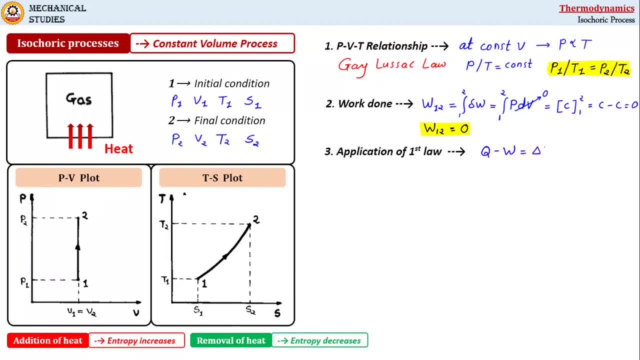 is equal to delta u. this is what the expression of first law of thermodynamics for non-flow process- and here work done associated with this process- is zero. so we get: ultimately q is equal to delta u. here q is equal to delta u. so please note here: heat transferred at constant volume to a substance. 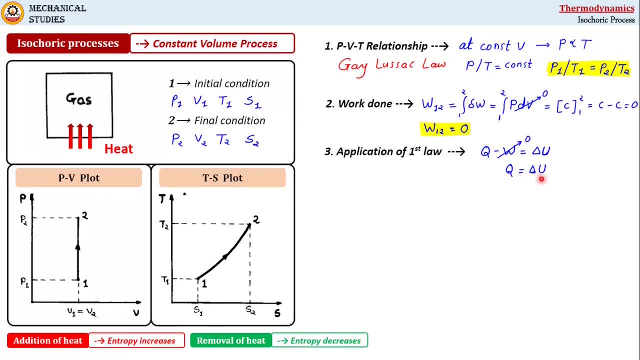 increases its internal energy. always okay. so the heat transferred amount of heat transfer is equal to change in internal energy. and change in internal energy can be calculated with an expression: delta u is equal to m c v delta t, m c v delta t. so this expression gives change in internal energy. so 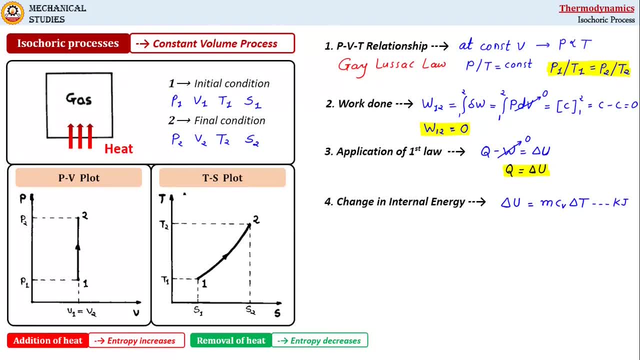 its unit will be kilojoule, whereas the change in specific internal energy or internal energy per unit mass will be expressed as small delta u. it will be equal to cv delta t, cv delta t. so we have already seen this in my previous videos: the expressions for internal energy and enthalpy. 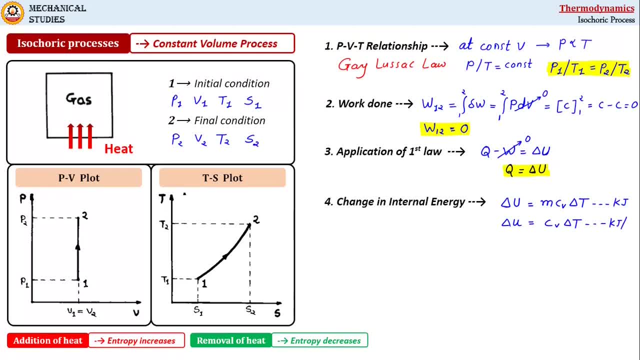 so here it's a internal energy per unit mass, so unit will be kilojoule per kg. okay, so with these expressions you can find out change in internal energy, delta u. okay, similarly, change in enthalpy can be calculated with expression: delta h is equal to m c p, delta t, m c p, delta t, where c p is. 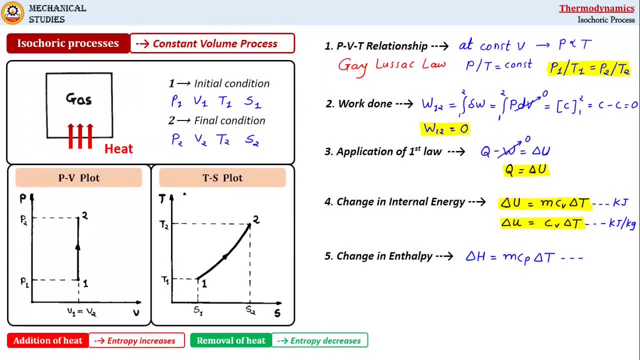 specific heat at constant pressure, and here its unit will be again kilojoule, whereas change in specific enthalpy, that will be small delta h, it will be given by c p delta t, c p delta t, and its unit will be kilojoule per kg. okay, so this is how you can find out change in. 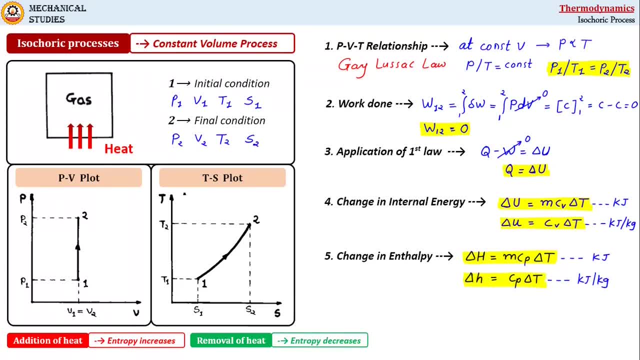 enthalpy, delta h. now please note here expressions for change in internal energy and change in enthalpy, that is delta u and delta h remains same everywhere for any kind of non-flow process. okay, and at the end i will introduce here expression for change in entropy, which is delta. 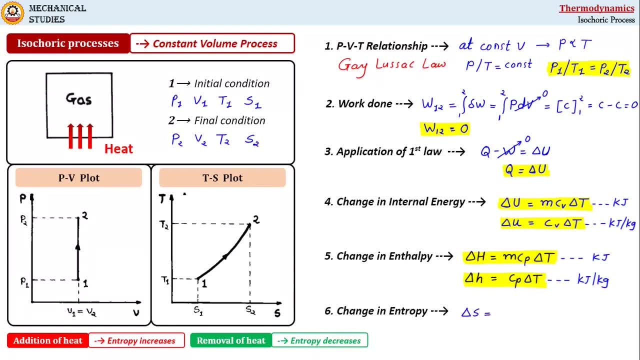 s is equal to m. the expression is delta. s is equal to mcv. log of remember. it's a log of t2 by t1, t2 by t1. so this is what an expression for change in entropy for isochoric process. so its unit will be kilojoule. 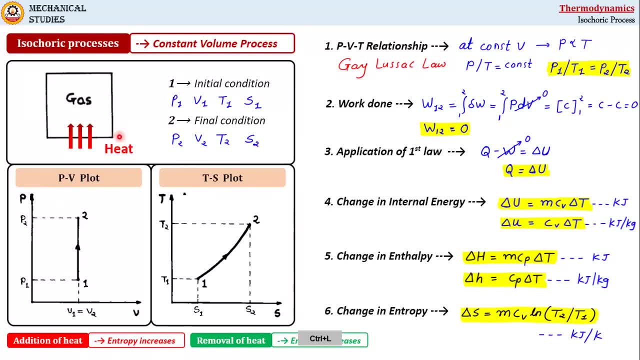 per kelvin. in this way we saw execution of constant volume, that is, isochoric process, pressure volume as well as temperature entropy, plot of this isochoric process. then we saw pressure volume, temperature relationship, work done associated with this process. then we saw application of first law and expressions of change in internal energy, change in enthalpy.